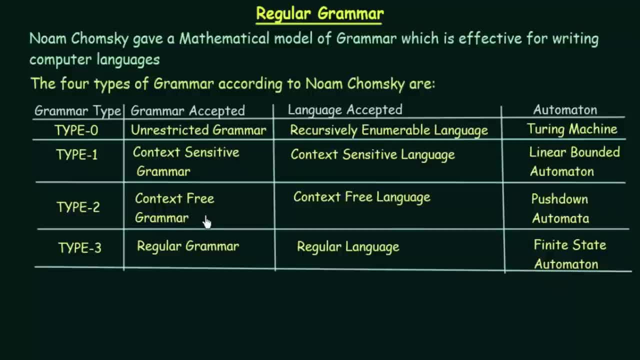 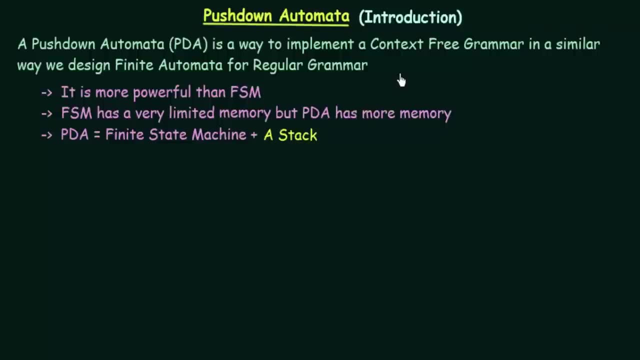 And in the past few lectures we have been studying about our context free grammar, which accepts the context free languages, And our push down automata is the automaton that is used for designing the context free languages. So let us see what are the main points that we need to remember about push down automata. 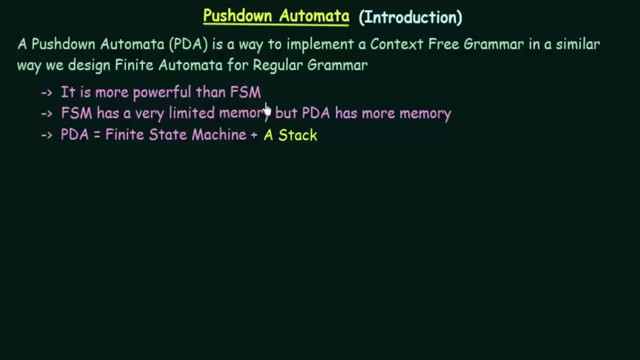 First one is it is more powerful than finite state machines. When we were studying about finite state machines, we studied that finite state machines has a very limited amount of memory, And we saw the limitations that we faced while designing finite state machines. There were certain grammars or certain languages that could not be designed using finite state machines due to their limited memory and other limitations. 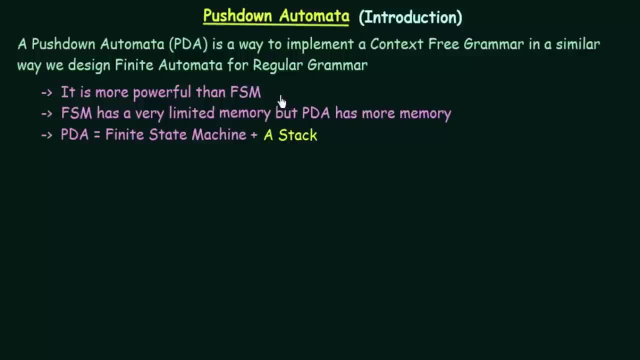 So this push down automata- it is more powerful than FSN. And those languages which could not be designed using FSN could not be designed using FSN, So this push down automata- it is more powerful than FSN- be designed using finite state machines can be designed using the push down automata and 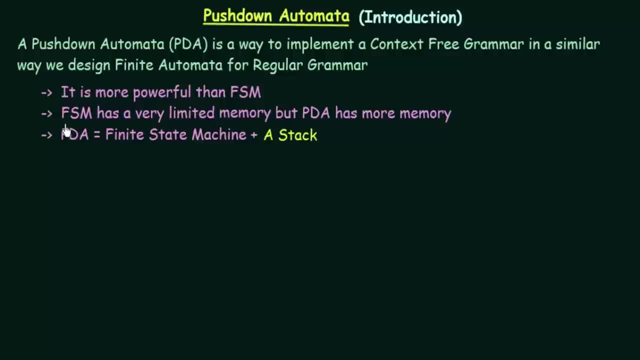 we will see how we can do them. And then the next thing is that FSM has a very limited memory, which we already studied. but push down automata has more memory. And then push down automata, it is equal to finite state machine plus a stack. 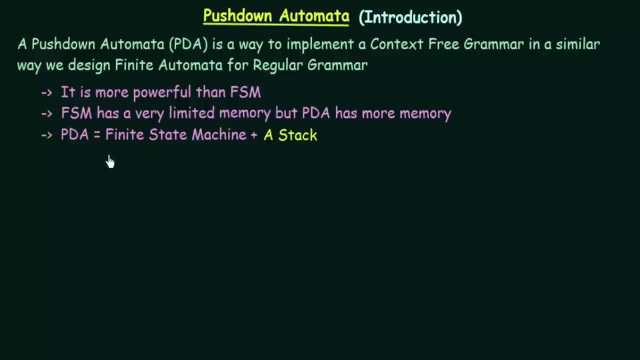 Now, what do I mean by this? is that the difference between a finite state machine and push down automata is that push down automata it consists of something like a finite state machine and the extra thing that we have in a push down automata is a stack. 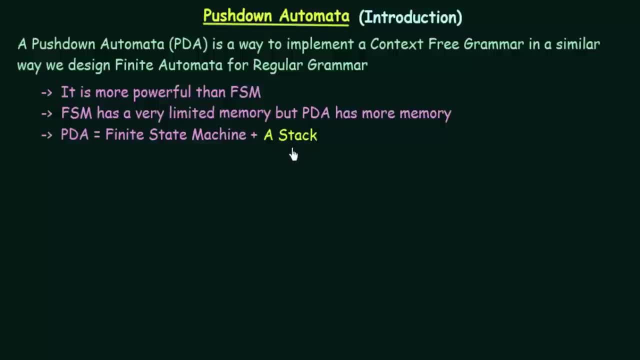 This stack has an infinite memory and this is the thing that facilitates the higher power of push down automata and this is what helps the push down automata to behave more powerful than the finite state machine. So we will see how this is And before that, 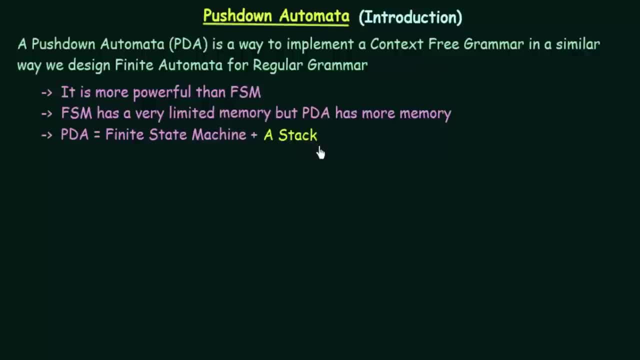 Let us see what is a stack and let us see what are the main operations that a stack can perform. If you have studied about data structure, you may know what a stack is, but let me just explain to you what it is over here. A stack is a way we arrange elements one on top of another. 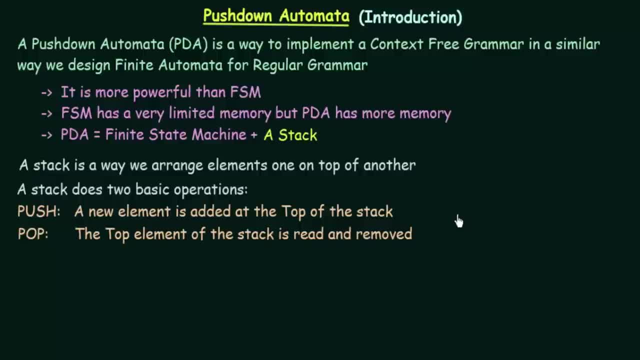 So a stack is a way we arrange elements, where we place them one on top of another, And a stack has two basic operations. One is known as the push operation, Which means a new element is added at the top of the stack, and another one is known 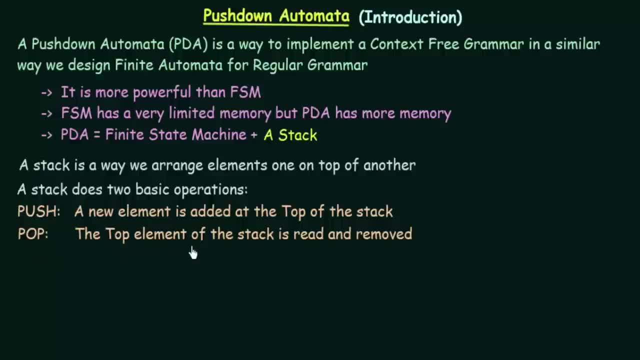 as the pop operation, where the top most element of this stack is read and removed. So let us try to first understand what these are. So here I have a diagram which depicts a stack. So, as I told you, a stack is a way where we arrange elements one on top of another. 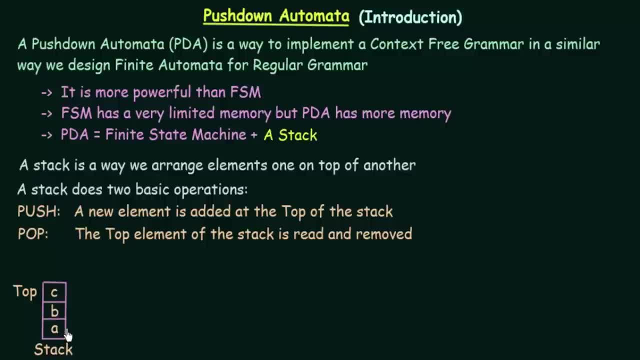 So here we see that we have three elements: a, b and c, and they are put one on top of another, So you can imagine this as a pile of them, a pile of books. When we arrange a pile of books, how do we arrange them? 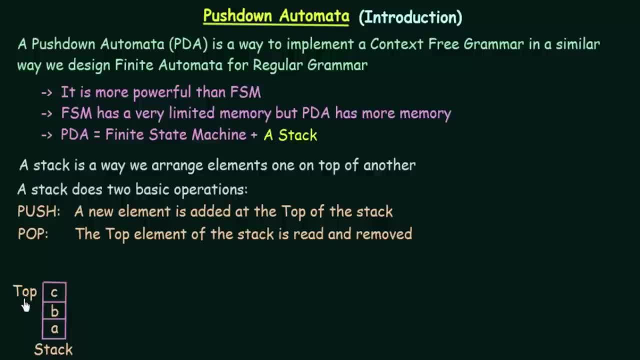 We put one book on top of another And the topmost element, that is denoted by top, and then let us see: how does the push and the pop operations work on a stack? So here I have my same stack and in order to understand push operation, 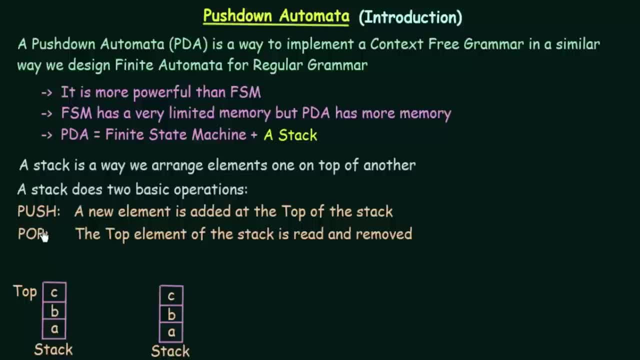 as I told you, imagine this as a pile of books, And push means you want to insert a new element. And when you insert a new book into your pile of books, where do you insert it? You have to always insert it on the topmost book. 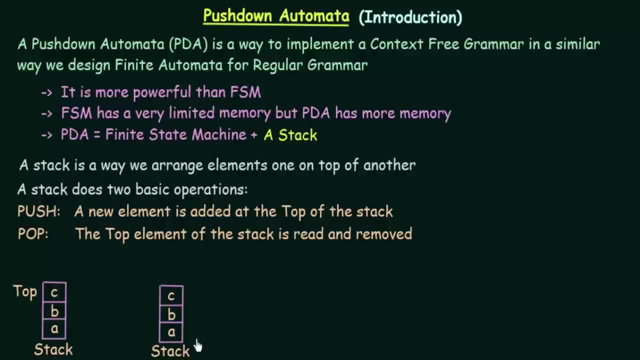 So when you do the push operation, what happens is that you are putting an element on the top of the topmost element. So here, when we push an element, let us say D, I am putting one more element on top of the stack. 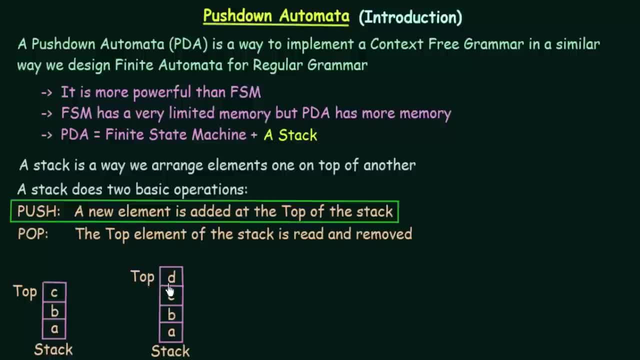 And now my top is denoted by the topmost element, which is D. Now let us try to understand what is the pop. Now, pop means to read and remove the topmost element of the stack. Now, if we are imagining it as a pile of books, 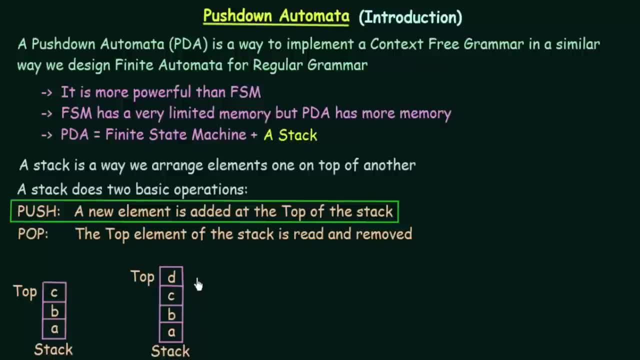 if you are arranging a pile of books like this and if you want to remove a book, from where do you remove? You have to start removing from the topmost. So popping means to remove the topmost element. So this is how you pop. when you perform the pop operation, 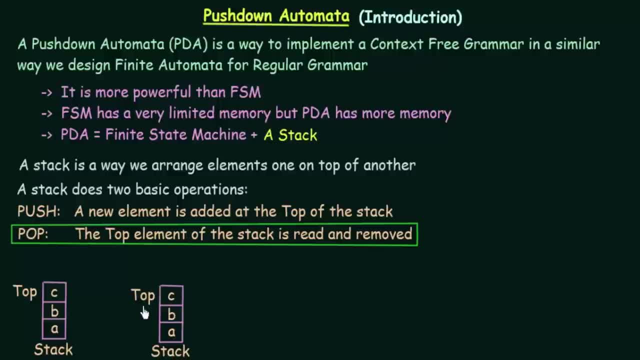 The topmost element, which was D, is removed, And now the new top, it is my element C. Now let us perform pop once more on this and let us see what happens. Now, if we perform pop once more, this is what happens. 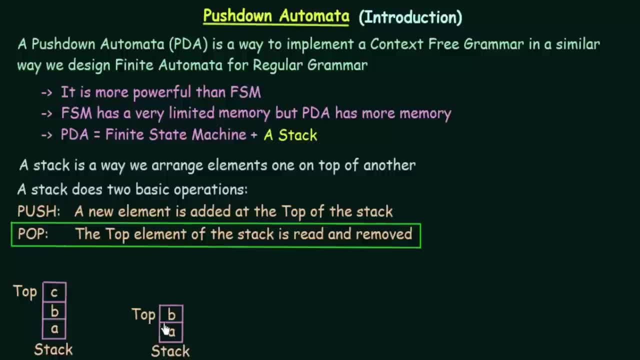 The topmost element, which was C. it is removed And then B becomes my topmost element. So those are the two basic operations that is performed by the stack Push and pop, And this stack will be used to implement our push-down automata. 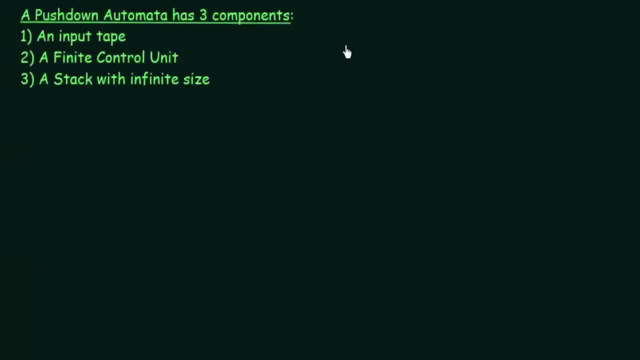 Now, as we have understood the operations of stack, let us now try to see what are the basic components of a push-down automata. So a push-down automata basically has three components. First one is an input tape which is like the input string. 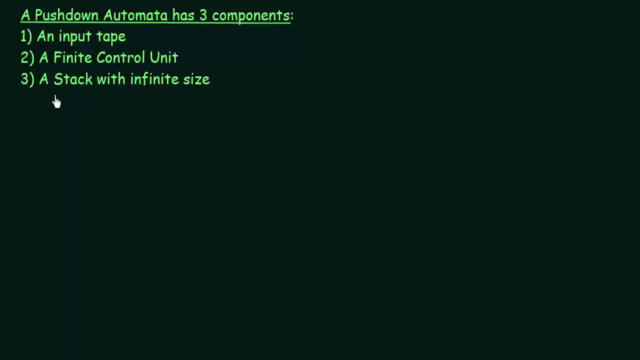 And then the second one is a finite control unit, And then the third one is a stack with infinite size. So here we have a diagram which depicts this. The input tape is shown here, which is like the input string that we have, And then the input string is given to the finite control unit. 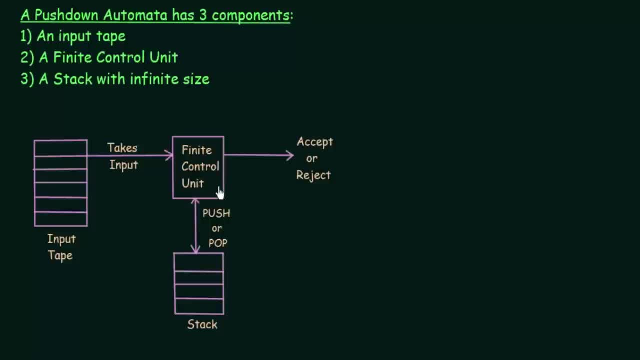 So the finite control unit takes the input And then we have a stack over here, which is the thing that we have in our push-down automata And this is the thing that we do not have in our finite state machine. So, based on the inputs, something will be pushed or popped from the stack. 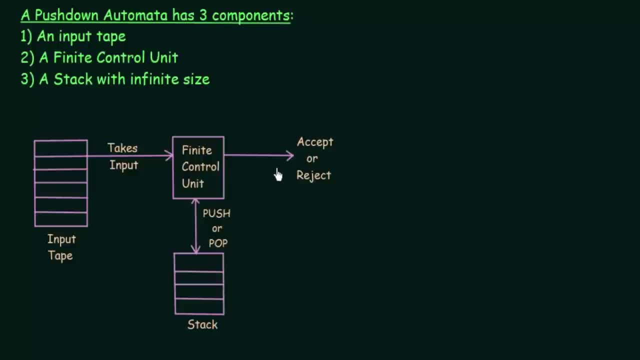 And finally we will have the string that will be accepted or rejected. Now don't worry, if you don't understand this- How the stack works and how a string will be accepted or rejected- all those things will be discussed later when we go in more detail into the push-down automata. 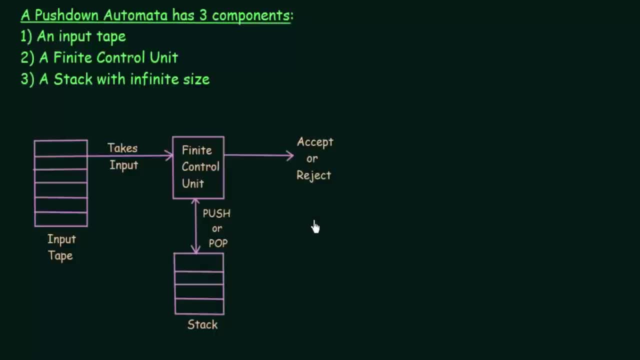 So this lecture was just an introduction to the push-down automata, Just to get you familiarized with the components of a push-down automata. And from the next lecture onwards we will be seeing in more detail about push-down automata And we will also see how we can formally define it. 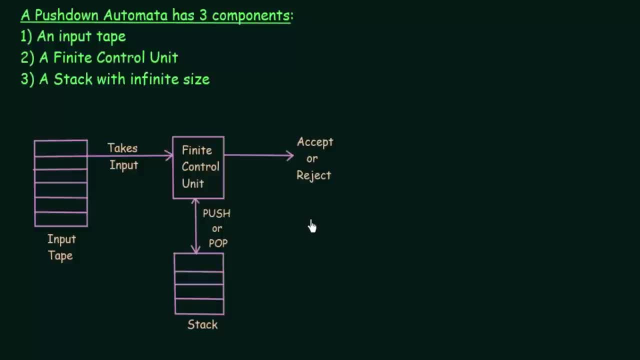 And we will also see how it actually works. So I hope this introduction was clear to you. Thank you for watching and see you in the next one.